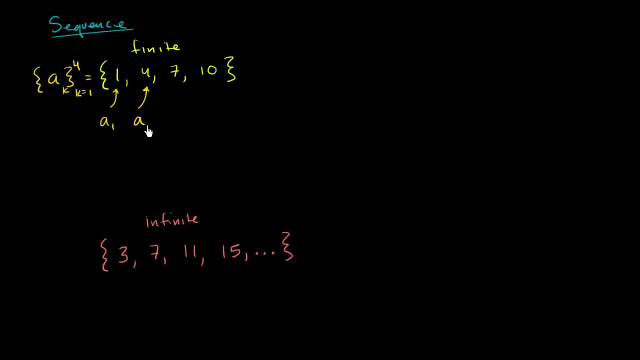 We would call that a sub 1.. This right over here would be the second term. We'd call it a sub 2.. I think you get the picture: a sub 3.. This right over here is a sub 4.. So this just says all of the a sub k's from k equals 1,. 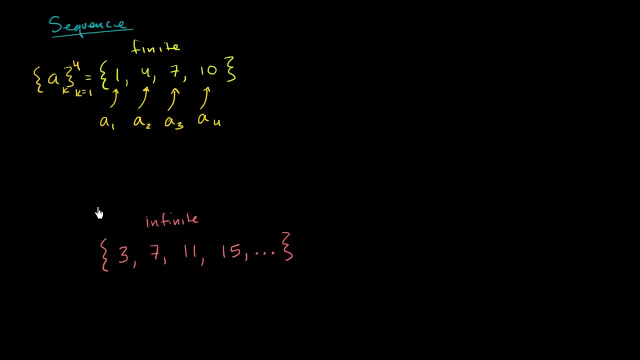 from our first term all the way to the fourth term. Now I could also define it by not explicitly writing the sequence like this: I could essentially do it, defining our sequence as explicitly using a function notation or something close to function notation. So the same exact sequence. I could define it as a sub k. 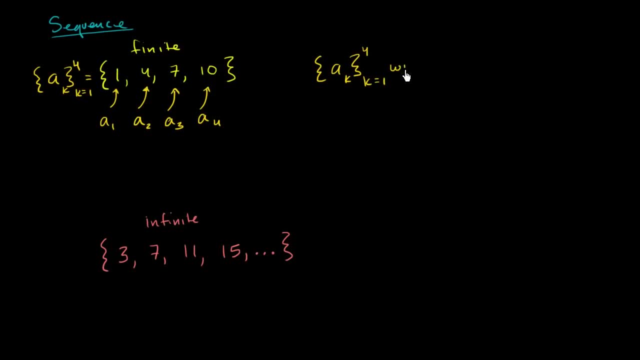 from k equals 1 to 4, with, instead of explicitly writing the numbers here, I could say a sub k is equal to some function. here It's a function of k. So let's see what happens: When k is 1, we get 1.. 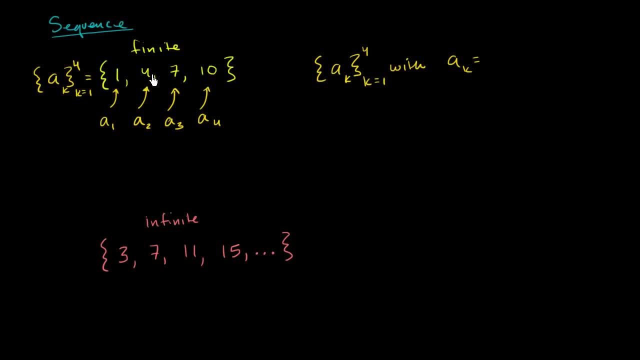 When k is 2, we get 4.. When k is 3, we get 7.. So let's see: when k is 3, we added 3 twice. Let me make it clear. So this was a plus 3.. 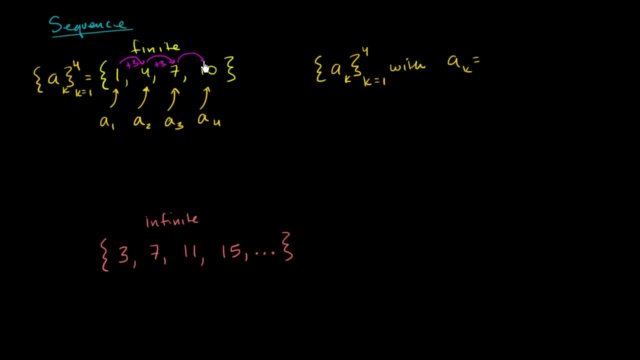 This right over here was a plus 3.. This right over here is a plus 3.. So, whatever k is, we started at 1, and we added 3,, 1 less than the k term, So we could say that this is going. 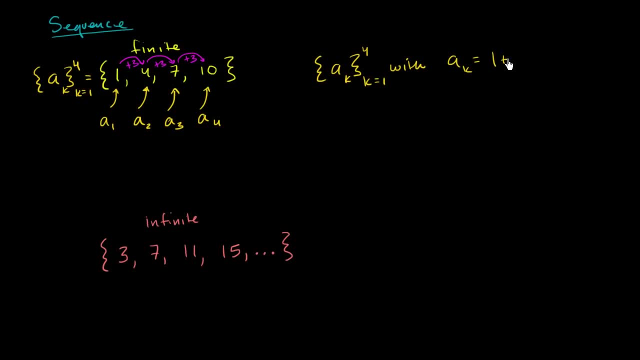 to be equal to 1 plus 1 plus k minus 1 times 3.. Or maybe I should write 3 times k minus 1.. Same thing 3 times k minus 1.. And you can verify that this works If k is equal to 1.. 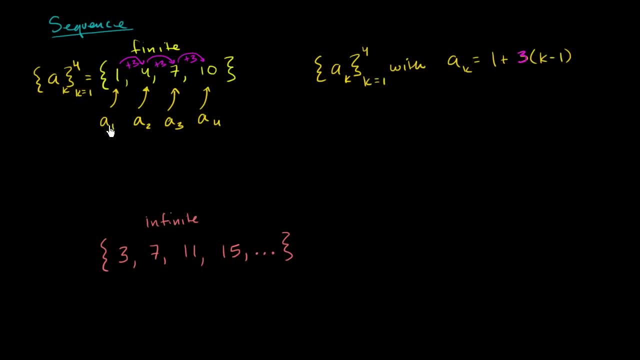 You're going to get: 1 minus 1 is 0. And so a sub 1 is going to be 1.. If k is equal to 2, you're going to have 1 plus 3, which is 4.. 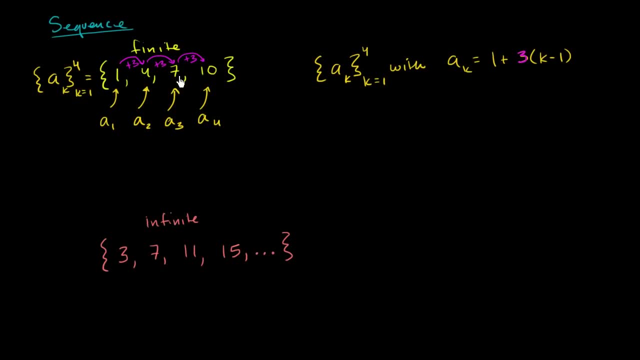 If k is equal to 3, you get 3 times 2 plus 1 is 7.. So it works out. So this is one way to explicitly define our sequence. with this function notation, I want to make it clear. I've essentially defined a function here. 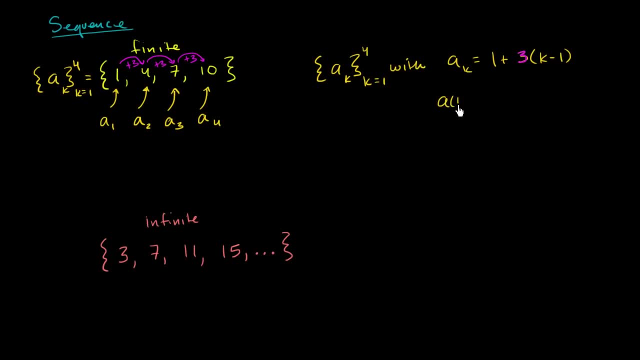 If I wanted a more traditional function notation, I could have written a of k, where k is the term that I care about. So a sub k is equal to 1 plus 3 times k minus 1.. This is essentially a function where an allowable input 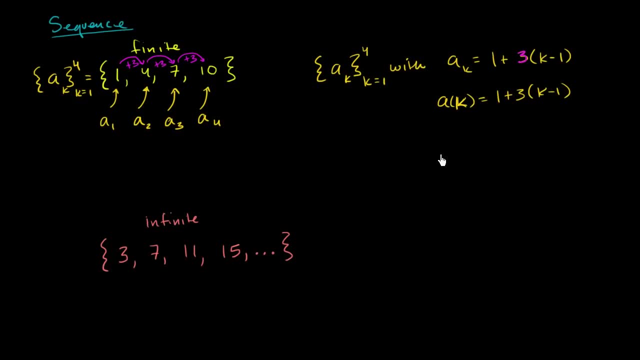 the domain is restricted to positive integers. Now, how would I denote this business right over here? Well, I could say that this is equal to, and people tend to use a, but I could use the notation b, sub k or anything else. 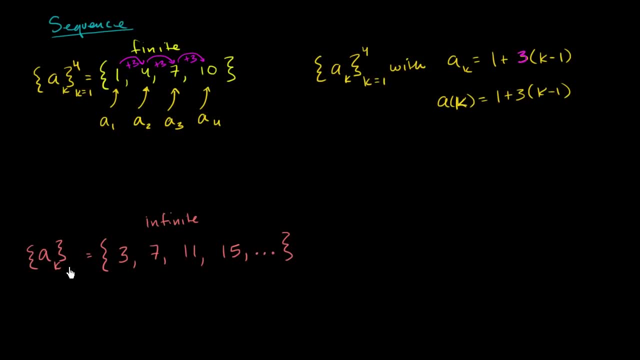 But I'll do a again, a sub k, And here we're going from our first term. So this is a sub 1.. This is a sub 2, all the way to infinity, Or we could define it if we wanted. 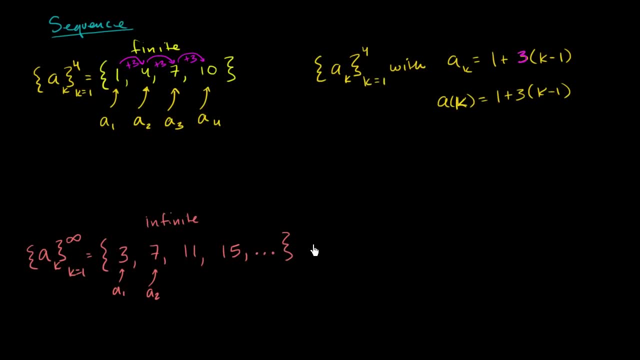 to define it explicitly as a function. we could write this sequence as a sub k, where k starts at the first term and goes to infinity with a sub, k is equaling. So we're starting at 3.. And we are adding 4.. 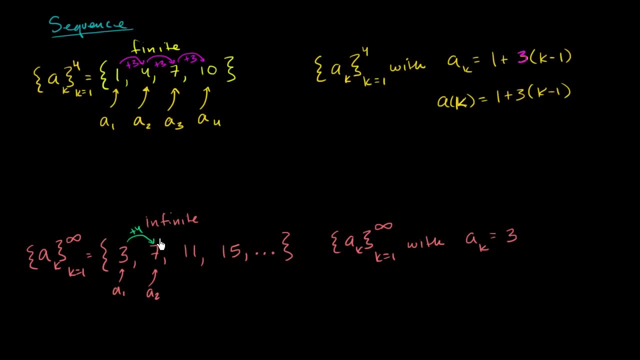 We're adding 4. One less time. For the second term, we added 4 once. For the third term, we add 4 twice. For the fourth term, we add 4 three times. So we're adding 4, one less than the term that we're at. 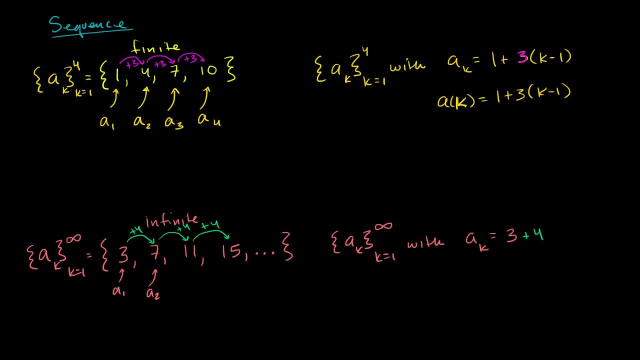 So it's going to be plus 4 times k minus 1.. 4 times k minus 1.. So this is another way of defining this infinite sequence. Now, in both of these cases I defined it as an explicit function, So this right over here is explicit. 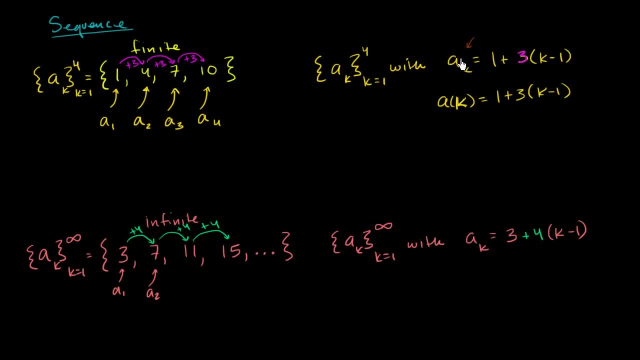 That's not an attractive color. Let me write this in: This is an explicit function, And so you might say: well, what's another way of defining these functions? Well, we can also define it especially something like this, like an arithmetic sequence. 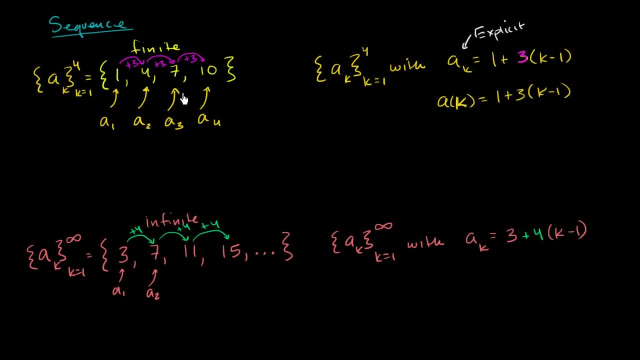 we can also define it recursively And I want to be clear: not every sequence can be defined as either an explicit function, like this, or as a recursive function, But many can, including this, which is an arithmetic sequence where we keep adding the same quantity. 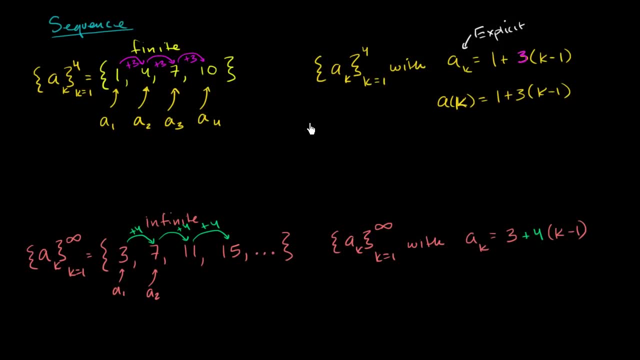 over and over again. So how would we do that? Well, we could also another way of defining this first sequence. we could say: a sub k, starting at k equals 1 and going to 4, with and when you define things recursively. 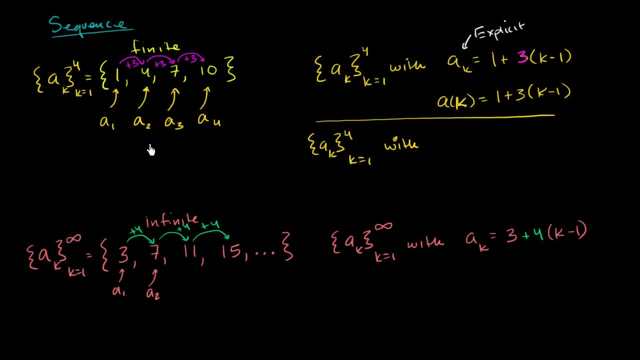 when you define a sequence recursively, you want to define what your first term is with a sub 1 equaling 1.. And then you can define every other term in terms of the term before it, And so then we could write a k plus. or let me write it this way: 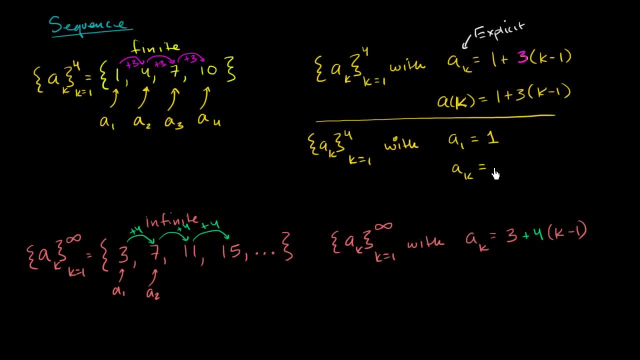 a sub k is equal to the previous term. So this is a sub k minus one, So a given term is equal to the previous term. Let me make it clear: this is the previous term plus the previous term plus in this case. 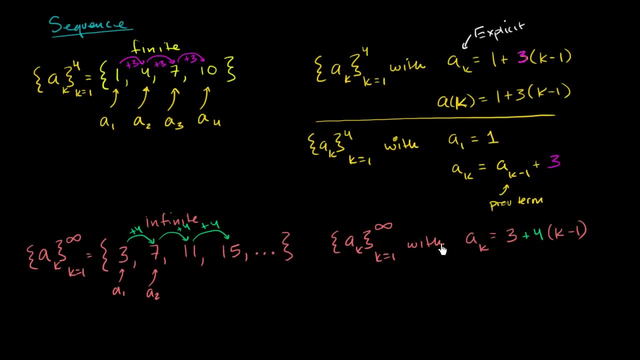 we're adding three every time. We're adding three every time. Now, how does this make sense? Well, we're defining what a sub one is. and if someone says: well, what happens when k equals two? Well, they're saying: well, it's gonna be a sub two minus one. 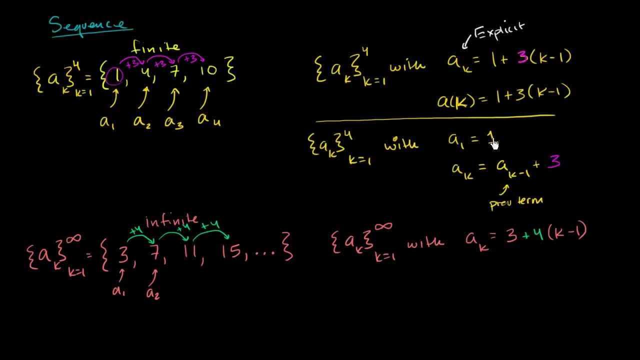 so it's gonna be a sub one plus three. Well, we know, a sub one is one, so it's gonna be one plus three, which is four. Well, what about a sub three? Well, it's gonna be a sub two plus three. 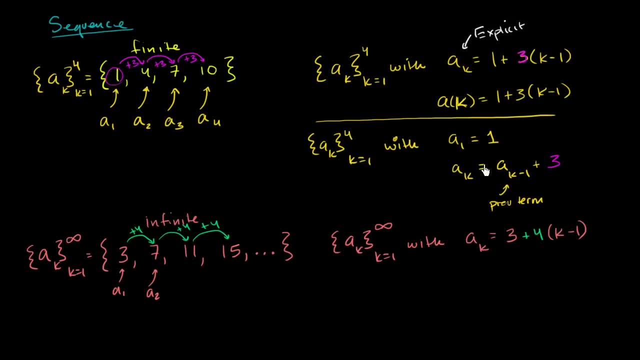 A sub two. we just calculated as four. you add three, it's gonna be seven. This is essentially what we mentally did when I first wrote out the sequence, when I said: hey, I'm just gonna start with one, I'm just gonna start with one. 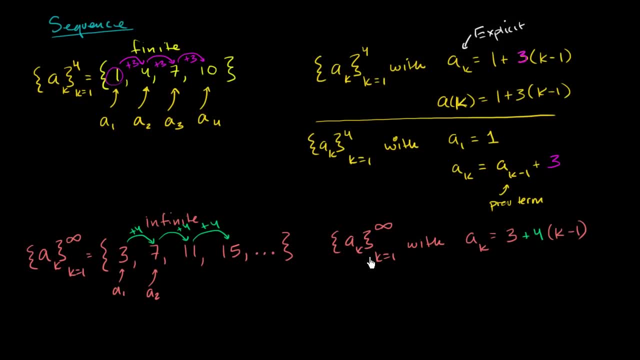 and I'm just gonna add three for every successive term. So how would we do this one? Well, once again, we could write this as a sub k, starting at k, the first term going to infinity. with our first term, a sub one is going to be three now. 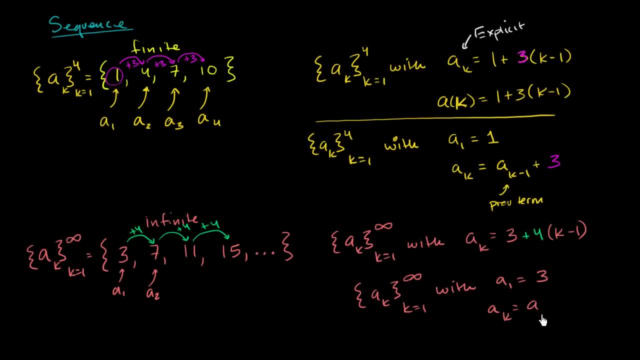 and every successive term, a sub k is going to be the previous term, the previous term, a sub k minus one plus four, Plus four, And once again you start at three, and then, if you want, the second term.